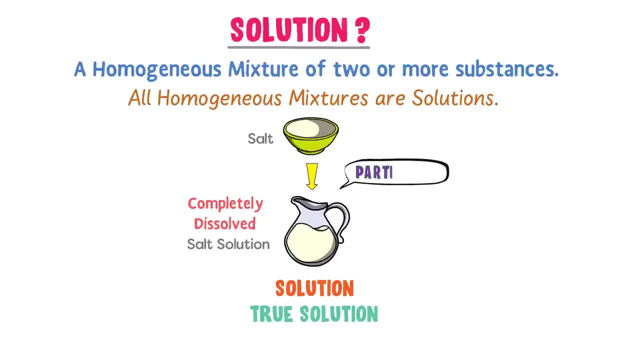 Here. let me ask you: Can you spot the particles of salt and water in this mixture? Well, you cannot spot the particles of salt and water in this mixture, Because both the salt and water particles are mixed in such a way that they form a uniform composition or homogeneous composition. 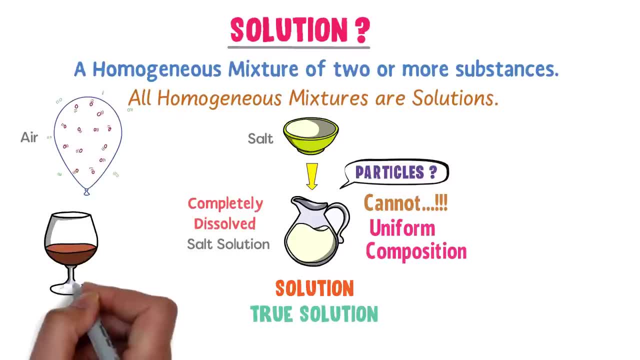 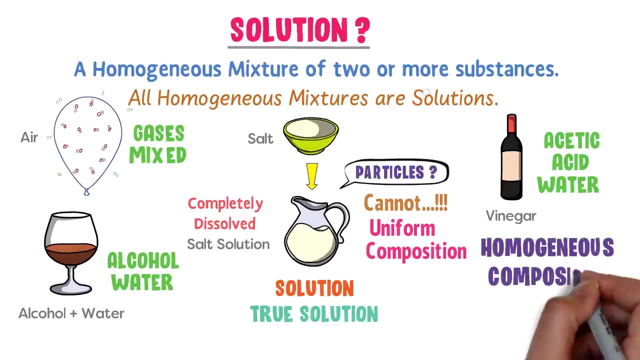 Some other examples of solution are air alcohol plus water and vinegar. In air, different gases mix together to form a homogeneous mixture. Alcohol plus water mix together in such a way that they form a uniform composition or homogeneous composition. In vinegar, acetic acid is dissolved in water and they also form a uniform composition or homogeneous composition. 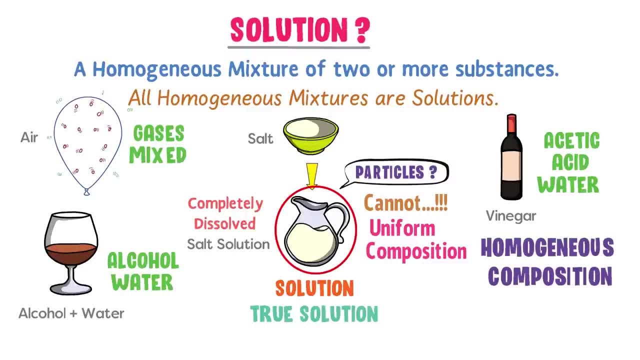 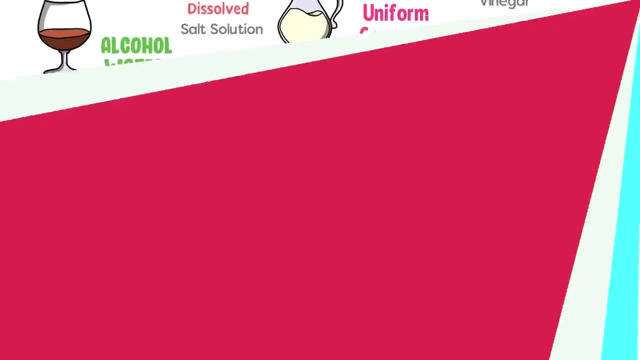 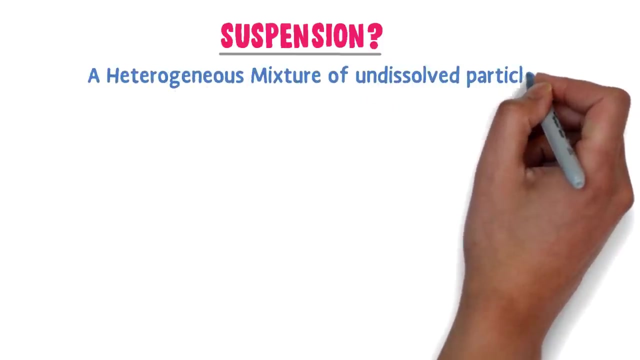 Thus, remember that a mixture is said to be a solution if its particles forms a homogeneous composition position. Secondly, in a solution, the particles are so small that we cannot spot them with naked eye. Now, what is suspension? Well, a suspension is a heterogeneous mixture of undissolved 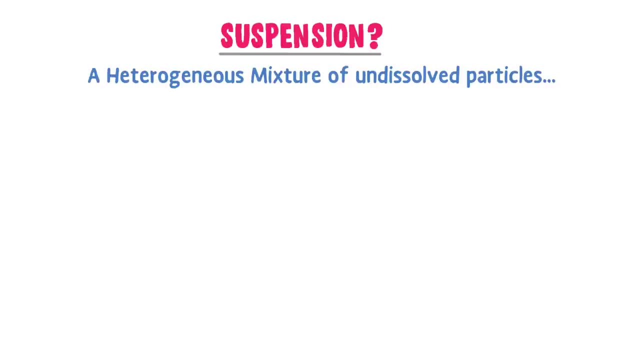 particles in a given medium. So all heterogeneous mixtures are suspensions. Let me repeat it: All heterogeneous mixtures are suspensions. For example, when we add mud or sand in the water, we get a suspension- Sand and water forms a non-uniform composition, a heterogeneous 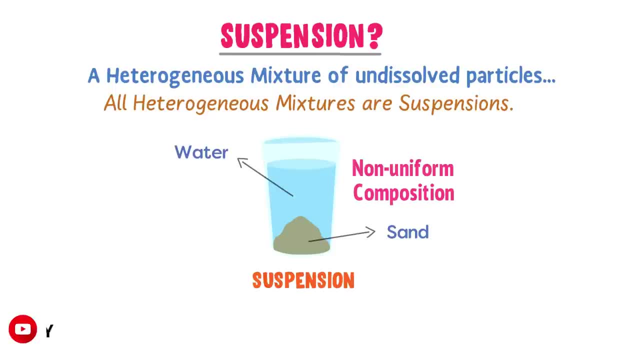 composition, Because if we left sand plus water for some time, sand settle down at the bottom and a clear layer of water appears at the top. We can spot large particles of sand and water at the bottom. So it is a heterogeneous mixture or suspension. Some other examples of suspension are oil plus. 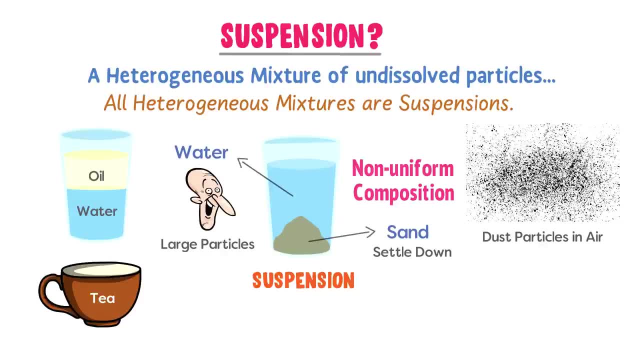 water, tea and dust particles in air. In oil plus water, we can spot the layer of oil and the layer of water. In tea, we can spot small particles of tea and a column of liquid, While we can spot small particles of water. we can spot small particles of tea and a column of liquid. 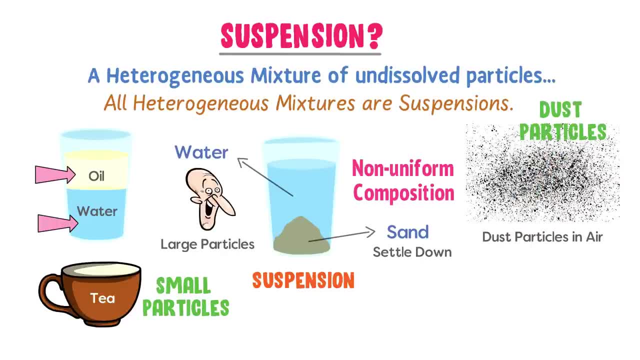 And we can also spot the dust particles in air. Just remember that a suspension is a heterogeneous mixture in which particles are large enough and can be seen with naked eye. Secondly, if suspension is left for some time, large or undissolved particles settle down at 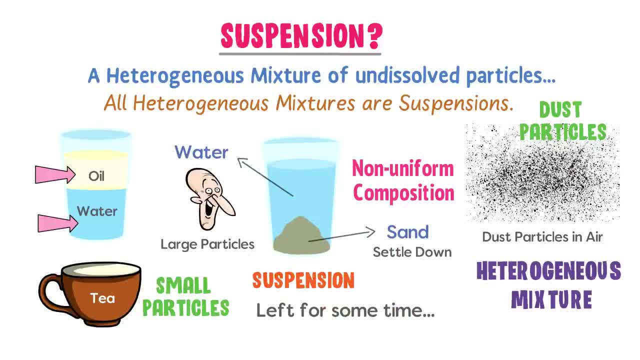 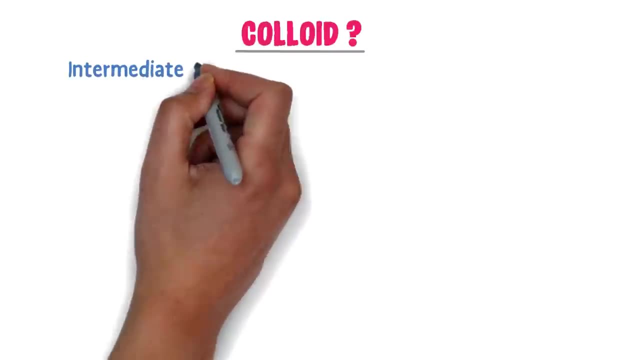 the bottom due to gravity. Let me repeat it: If suspension is left for some time, large or undissolved particles settle down at the bottom due to gravity. Now, what is a collide? A collide is intermediate state between a solution and suspension, For 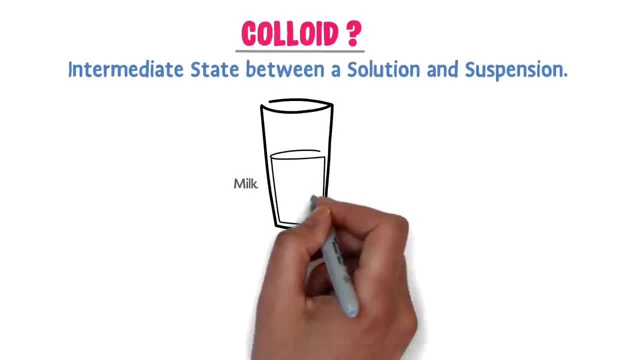 example, consider some milk. We know that milk contains globes of butter fat suspended throughout the liquid. So milk is a collide Because the particles of milk are intermediate in size between both of a solution and suspension. even if a collide or milk is allowed to stand, 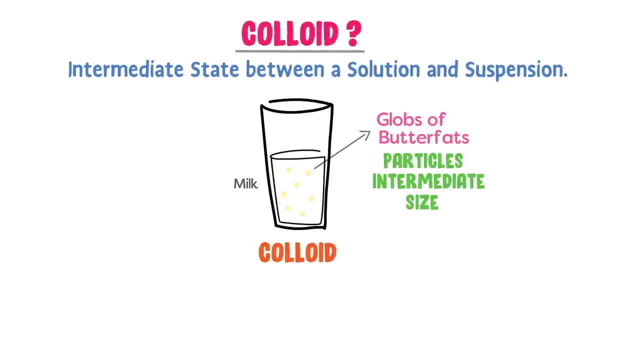 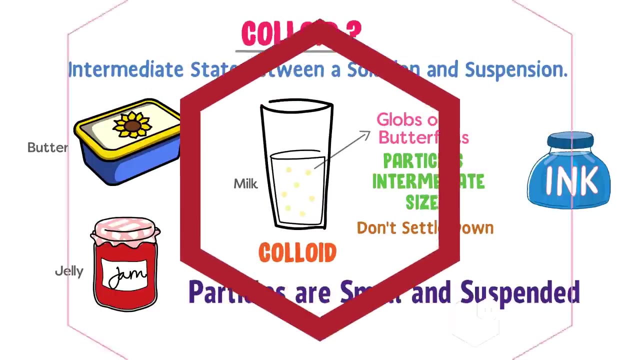 for some time the particles of collide or milk will not settle down. Some other examples of collides are butter, jelly, ink – and if these collides are OK, particles are small and suspended, So milk is suspended. Secondly, these particles are interlinked. Mini particles are thin and bulky. 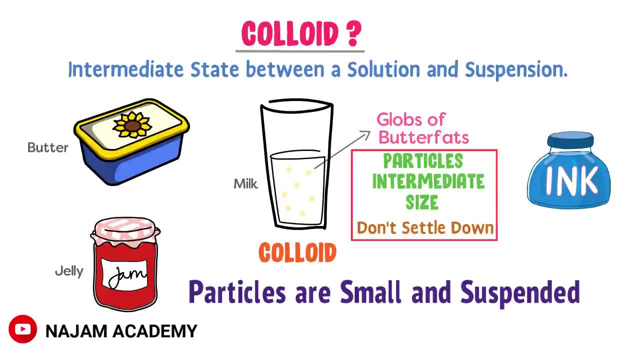 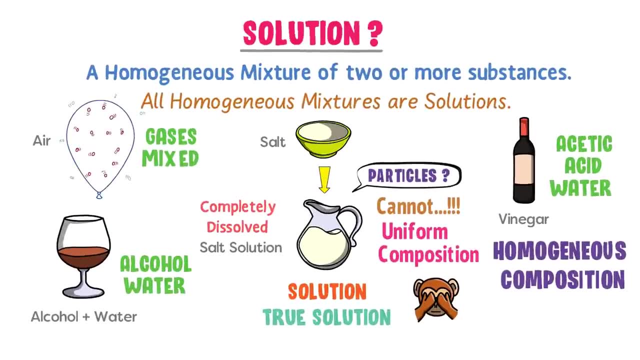 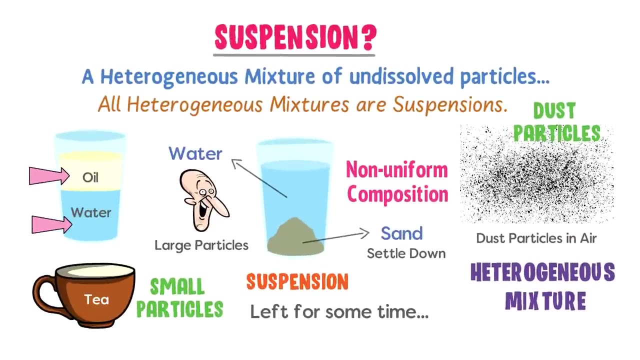 Secondly, these particles of collide will not settle down at the bottom, even if they stand for some time. Until now, we learned that a solution is a homogeneous mixture which forms a uniform composition and we cannot spot the particles in it like salt solution. Secondly, we learned that a suspension is a heterogeneous mixture which forms a non-uniform 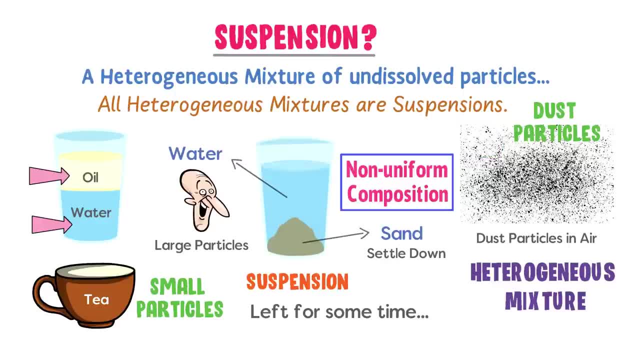 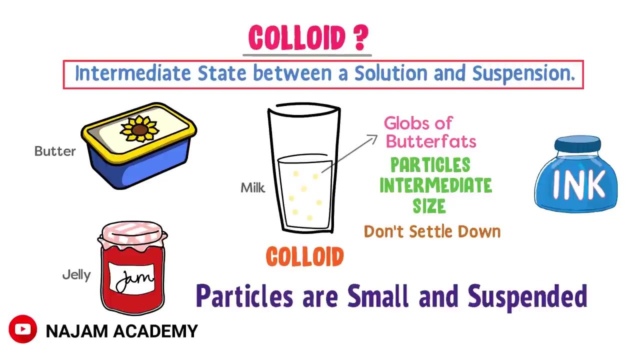 composition and we can spot the undissolved particles in it. Also, if suspension is allowed to stand for some time, its big particles will settle down at the bottom due to gravity. For example, sand plus water forms a suspension, While we also learned that the intermediate state of a solution and suspension is a collide.